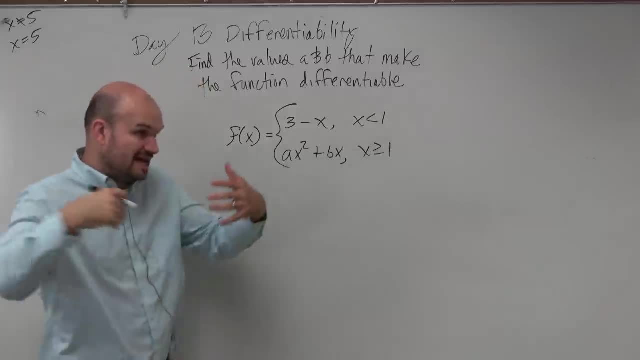 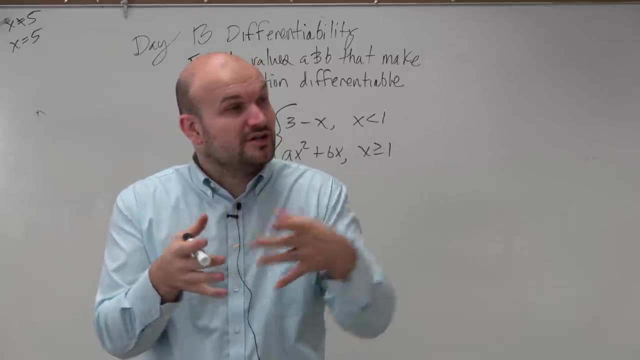 So we want to find the values that a and b make the function differentiable. Now the last example. the reason why I showed you continuity and differentiability- that's very nice- is because I want to show you there's two ways that we can make sure that something is differentiable. 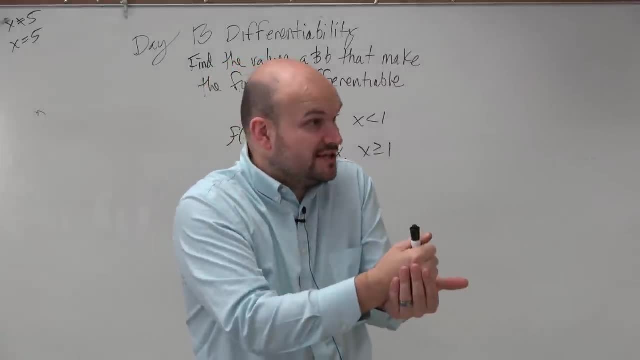 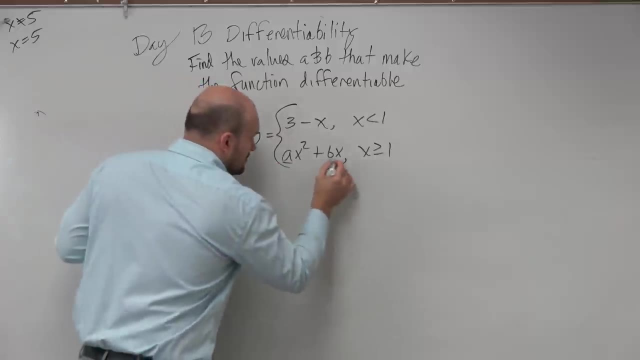 It has to be continuous and it has to be obviously. you have to find the derivative on the left and right side have to be the same when the piecewise function. So since we have two variables, we know we need two equations. 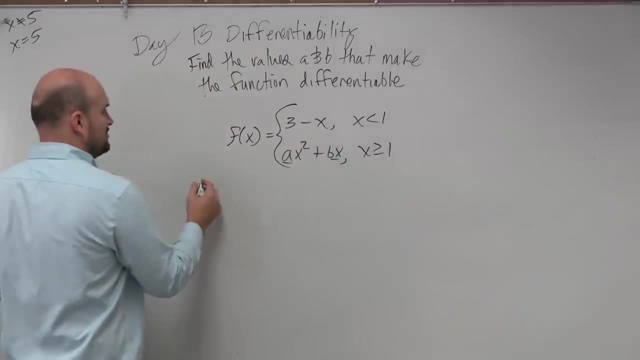 So let's test both of those. So let's test both of those, which, in this case, is going to be actually. I'm going to do that last example. I'm going to do one more example for you, because I think I'll drive home that point. 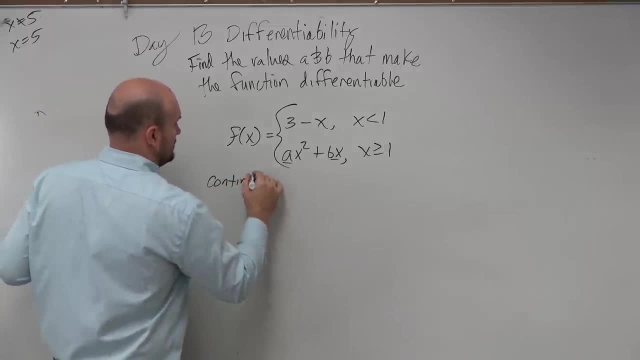 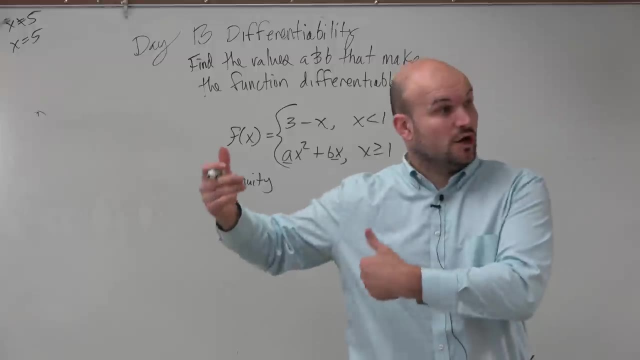 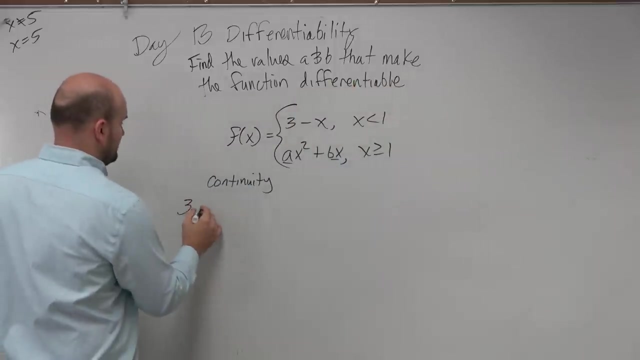 So let's check continuity. So if I want to check continuity again, I'm not checking continuity at 5. I want to check continuity at 1, because we know this is not a whole correct. So we only want to check continuity at where they could dissect or not meet. 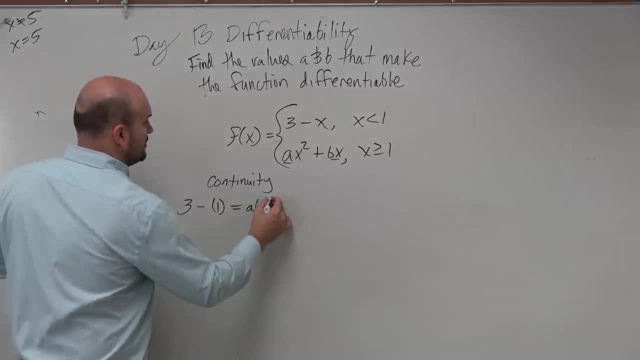 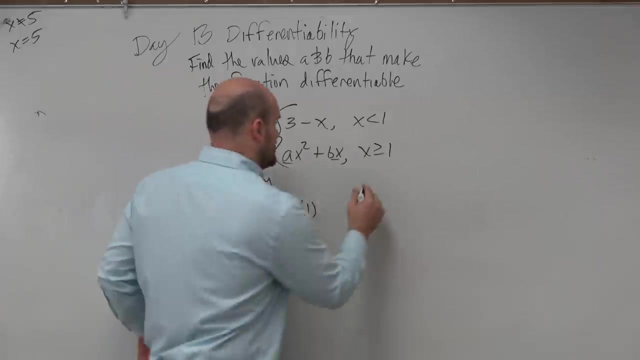 So we're going to check continuity here at a times 1 squared plus b times 1.. Would you guys agree with me on this? So we do this: we get 2 equals a plus b. OK, One equation. The next thing we want to do is check differentiability. 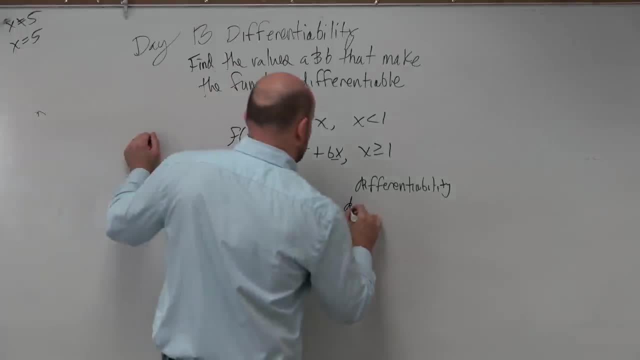 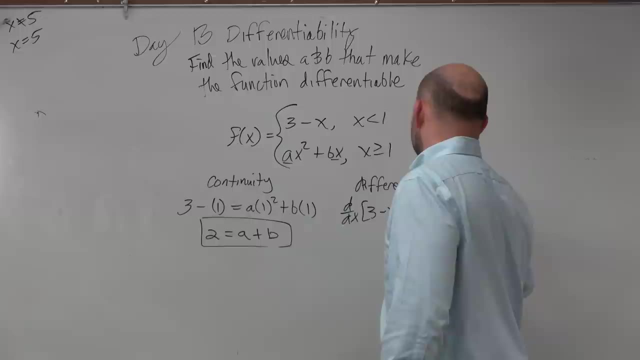 So to check differentiability, what we want to do is take the derivative d over dx of 3 minus x and have that equal to d over dx of ax squared plus bx. Now it's very important for us to remember what do a and b represent here. 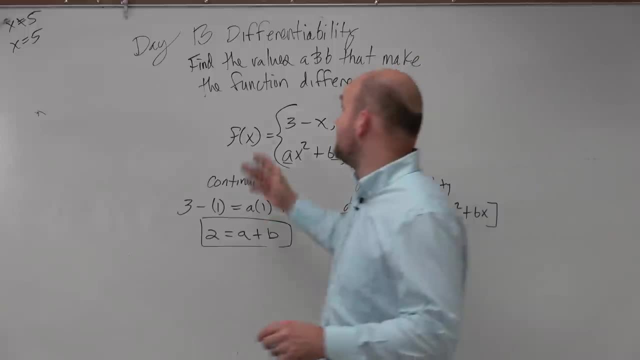 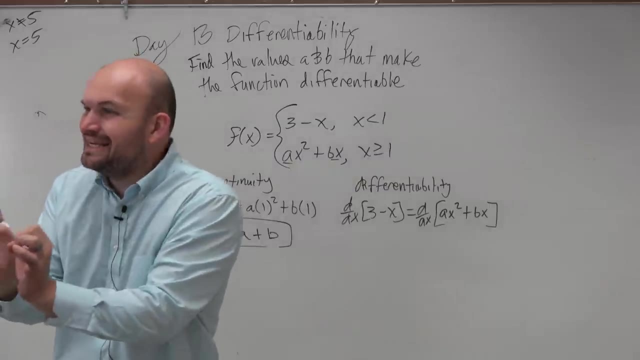 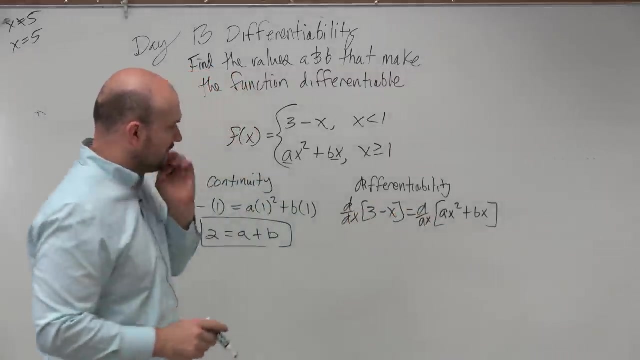 a and b are supposed to be representing values, but they're actually constants in this equation. right, They're not variable, They are unknown variables, but they're representing constants. That's important because when we're taking the derivative here, first of all we're taking differentiability at x equals 1.. 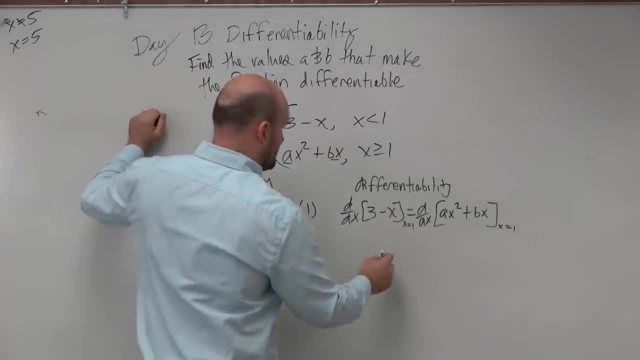 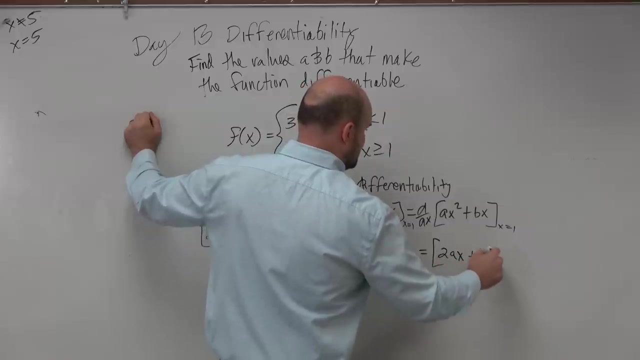 OK, So what we're going to do is take the derivative and then evaluate. So therefore, here I'm just going to have negative 1.. That's x equals 1, which is the same d over dx. here is going to be 2ax plus b. 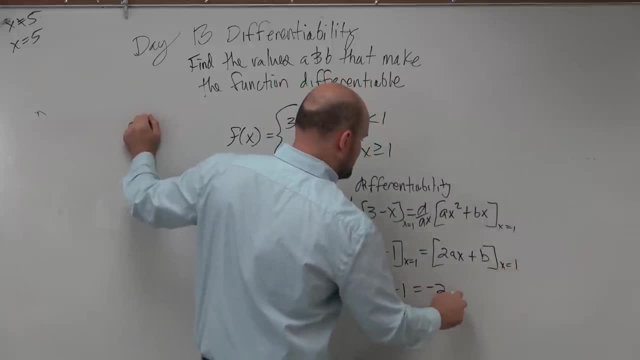 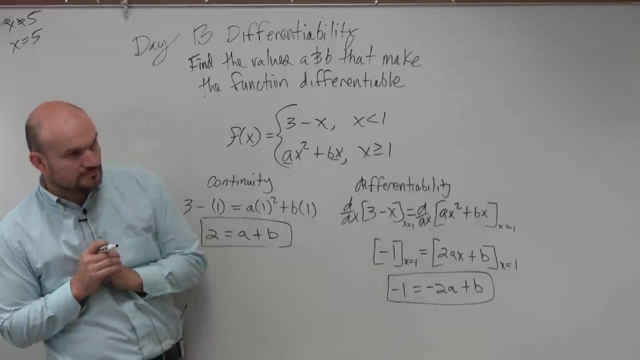 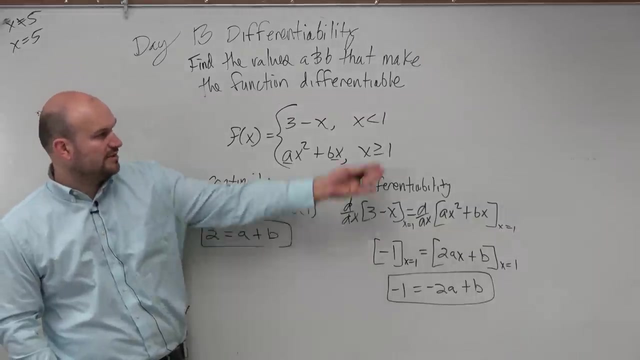 So therefore I get negative. 1 is equal to negative 2a plus b. Does everybody see what I did? I took the derivative and then evaluated the derivative at 1.. OK, So I'm going to take y1,, because that's. 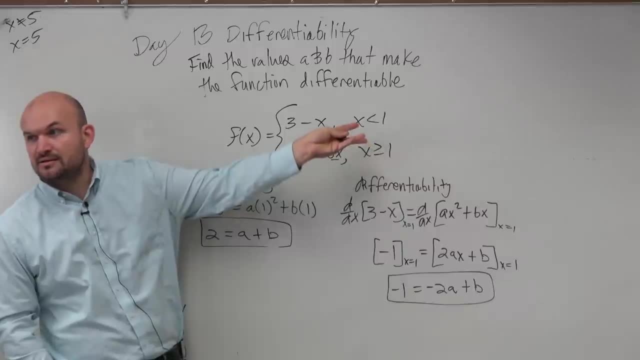 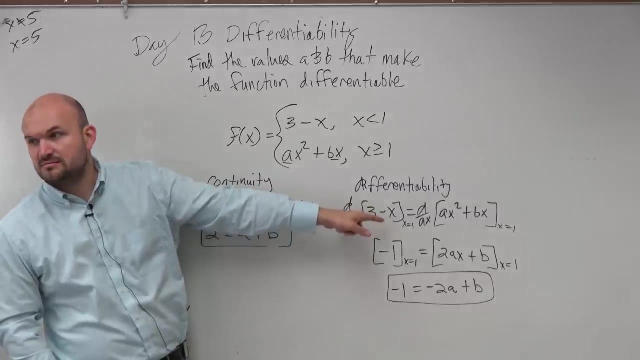 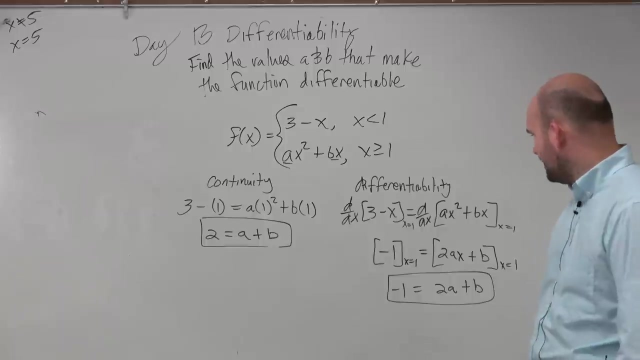 where I want to test the derivative on the left and right-hand side. This one: Yeah, So just the derivative of 3 minus x. I don't know That should be a positive right. Yeah, So it should be 2a plus b. 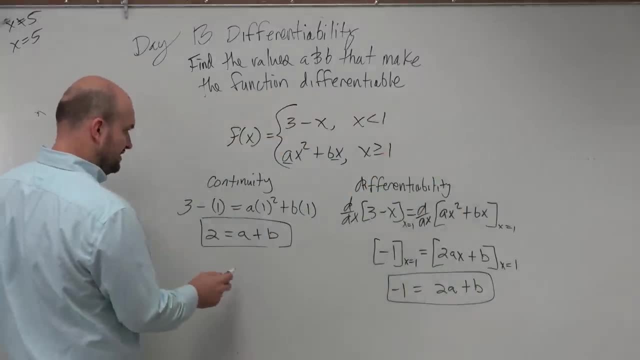 So now we have a systems of equations. So thankfully your Algebra 1 teacher, OK, Helped you guys out with systems of equations- or maybe not- So you can do elimination, You can do substitution, whatever you can. You can use a multiple. 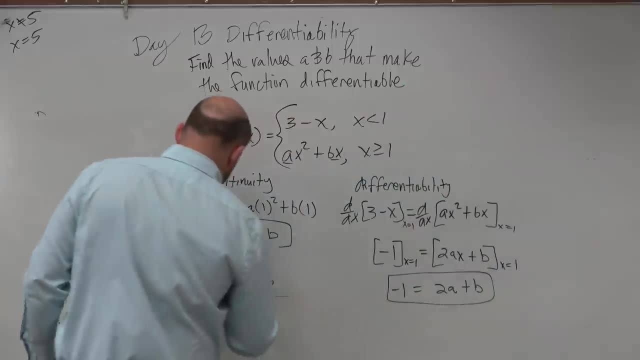 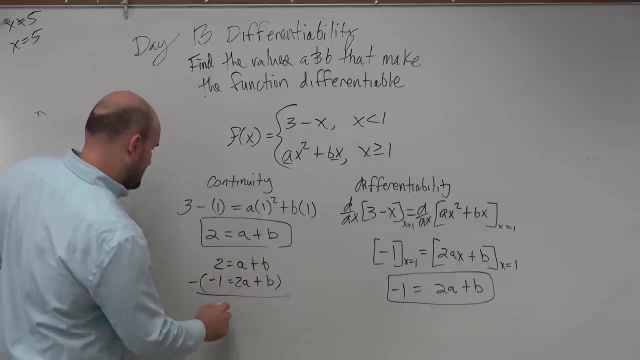 I see that I can quickly subtract the b's, So I'm going to use parentheses and subtract the rows. That will get rid of my b's. So 2 minus a negative 1 is going to be 3 equals a minus 2a. 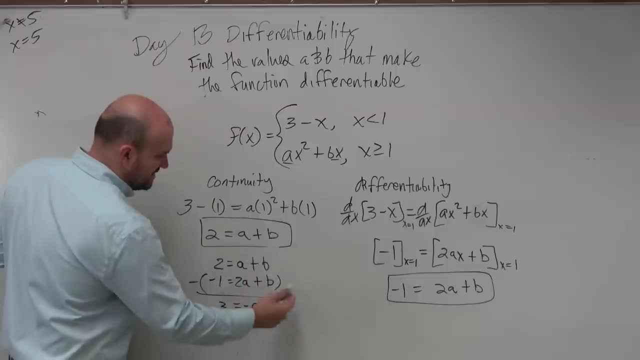 is going to be a negative a, And then that obviously b minus b. it just goes to 0. Divide by negative 1, divide by negative 1. I can say a is equal to negative 3. Now I know what a is. 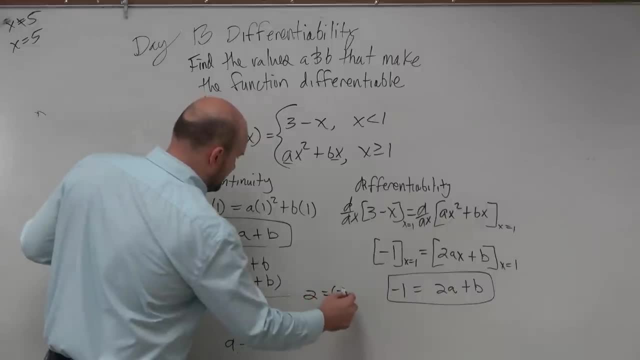 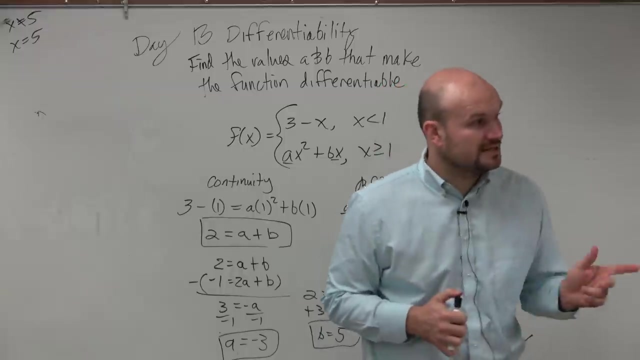 Let's find b. So I do: 2 equals negative. 3 plus b. Add 3, add 3, b equals 5.. So the values that make the function differentiable are going to be negative: 3 and 5.. Yes, 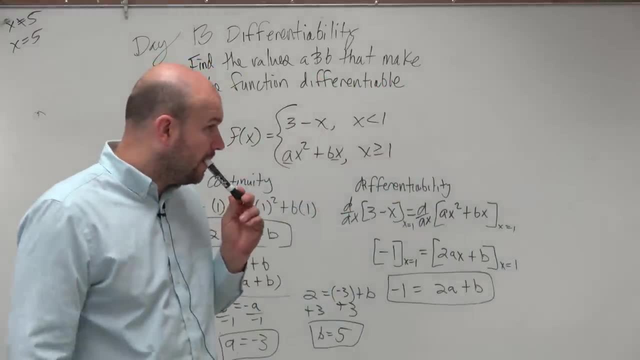 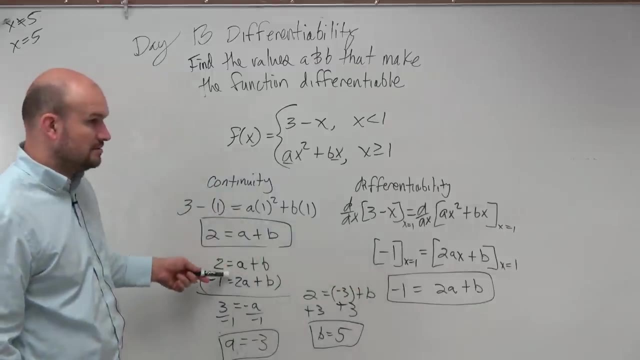 So 2 equals 2.. Huh Yeah, 2 for a and 2 for b. OK, So where did we, Where did we differentiate from each other Here? Do we have the same equations? Do we have the same derivative? 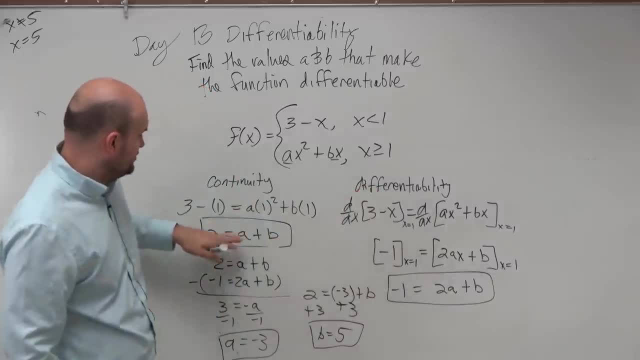 I mean, I'm not saying I don't know. Did I make a mistake? You made a mistake. I'm trying to say: where do we? Did you get that equation? Yes, Did you get that equation? Yes, That didn't sound as confident. 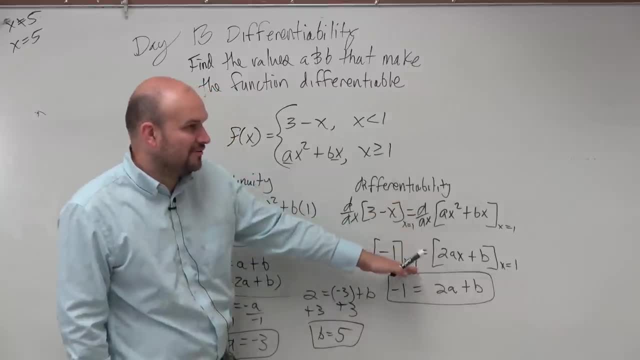 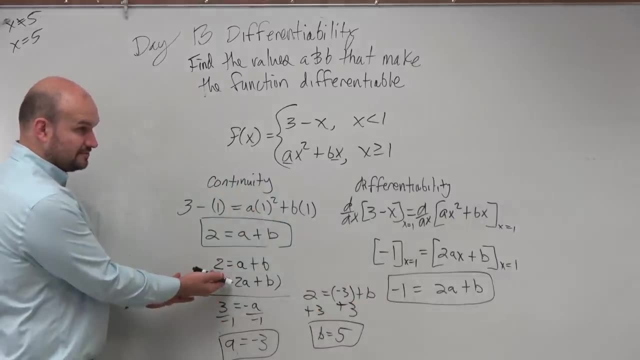 I mean it could be represented differently. Did you take the derivative and plug in 1?? Yes, OK, But you didn't get this. Oh, yeah, OK, So you have the same system of equations. I have the 2 equals a plus b, but I did it in a different way. 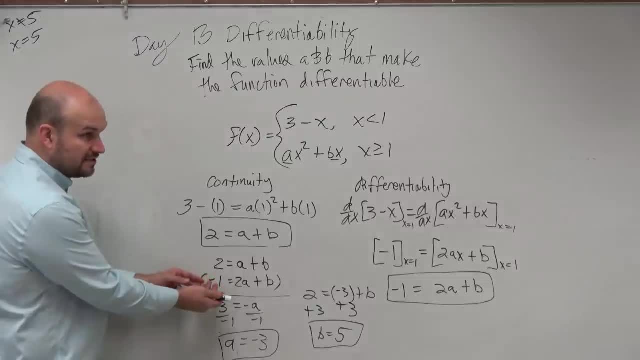 OK, How did you solve this system? So you have the same system, but you solved it differently. I got a equals 2 minus b, because I subtracted the b from each side, so it would be 2 minus b over a. 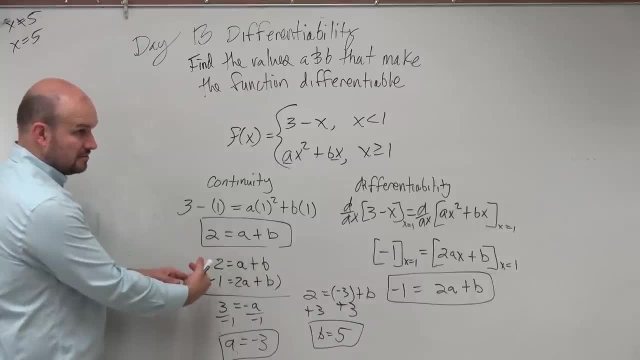 OK, So you subtracted b. and then you did what? substitution? Yeah. then you plugged a into that equation. I mean the a, yeah, Well, no, Say you subtracted b on both sides. OK, OK, OK. 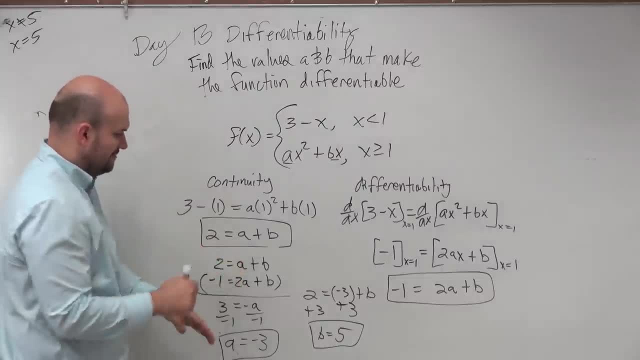 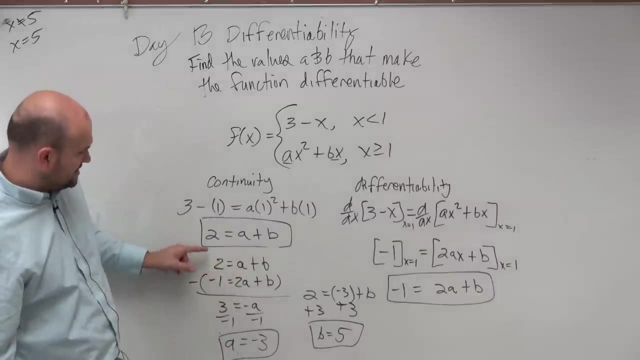 Yeah, Never mind. OK, Well, let's double-check my work, see if I made a mistake, and then we'll look at yours to see if maybe you made the mistake on something you did. Let me just double-check, because I make mistakes all the day. 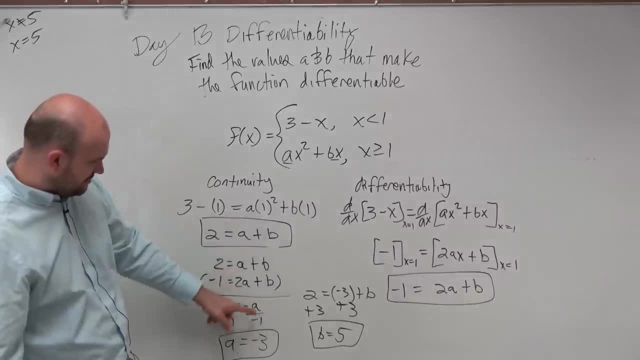 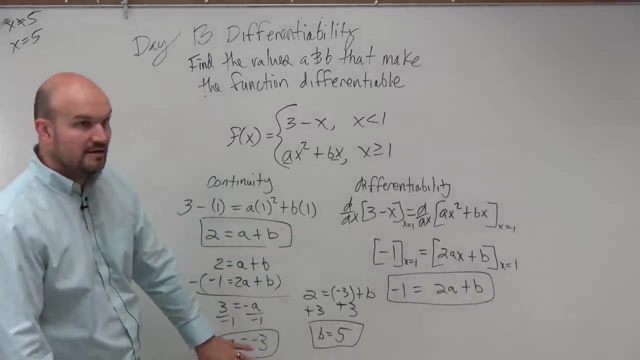 2 minus negative 1 is 3.. a minus 2a is negative, a 0 divided by negative 1.. I feel good with my work, So you might have just made a simple mistake when you did it a different way, which is perfectly fine. 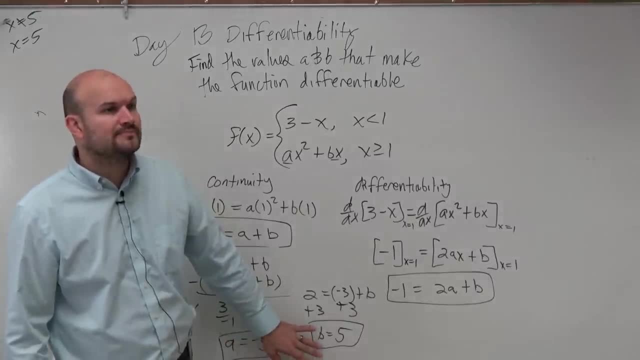 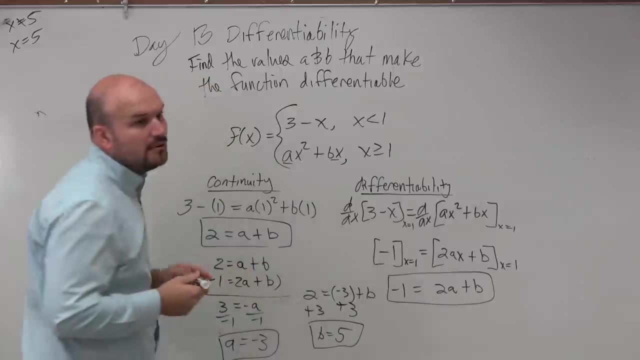 Anybody else raise their hand? that had another question, Sir. Yeah, So when you're making your system, do you want to do that before or do you do it later? Basically, Yeah Well, remember the first example I did. We were trying to see if something was differential.